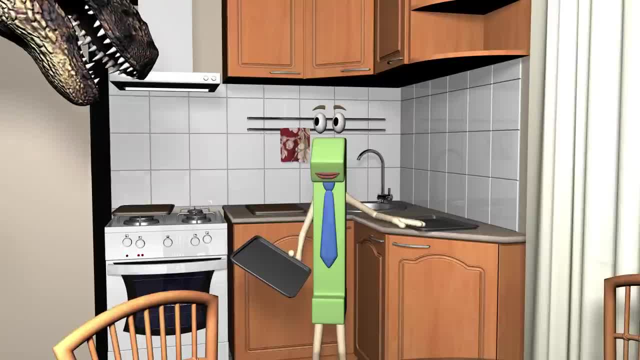 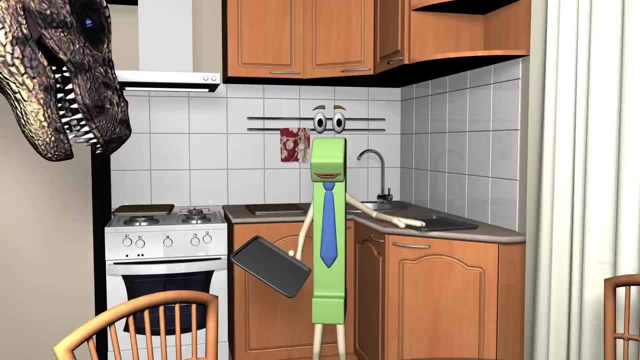 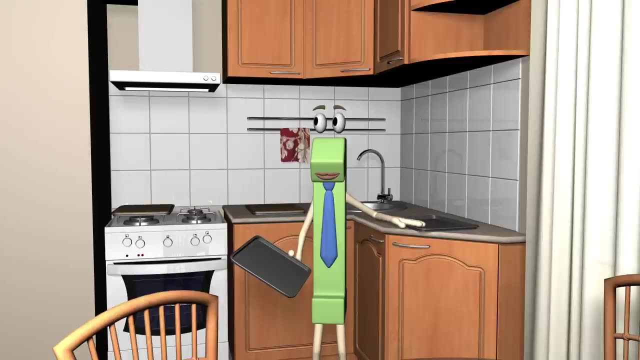 Hey kids, Sorry about that, I'm cooking brownies for my friend T-Rex. They have a party each year called the Equivalent Fraction Party. It is my job to bake the brownies before they get too hungry. Hey, I'm coming, Just give me a minute. Wait. do you smell something? Uh-oh, I think I burned the. 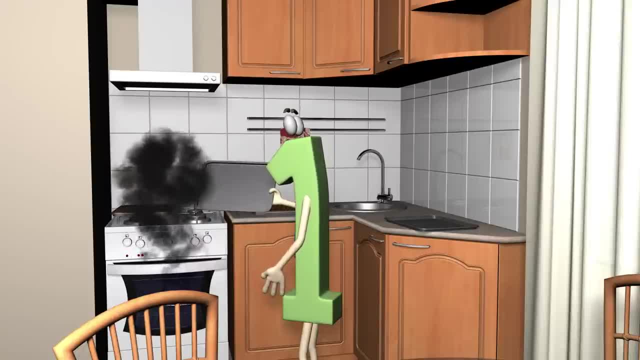 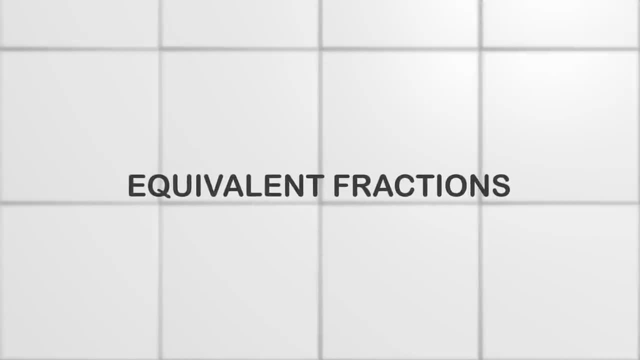 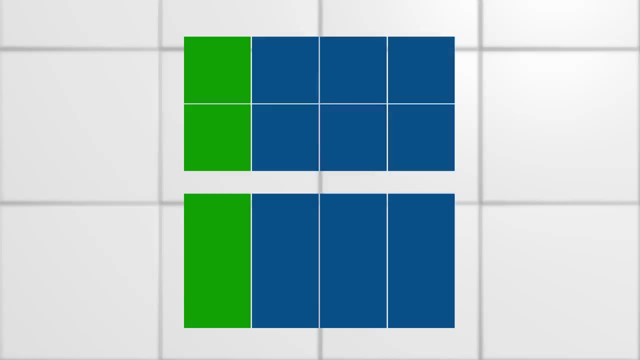 brownies. Why don't you guys learn about equivalent fractions while I fix this mess? Today we are learning about equivalent fractions. The word equivalent really just means equal or the same. Here we have two rectangles. We can see that they are exactly the same size but are divided up. 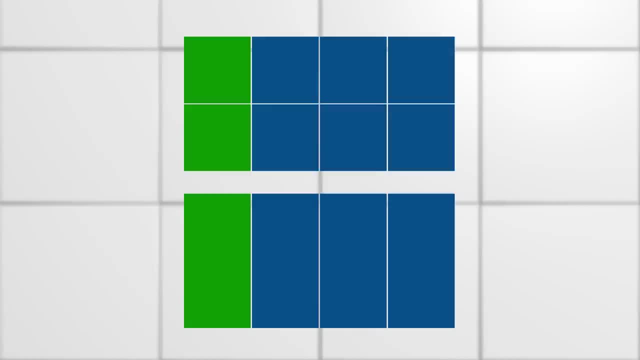 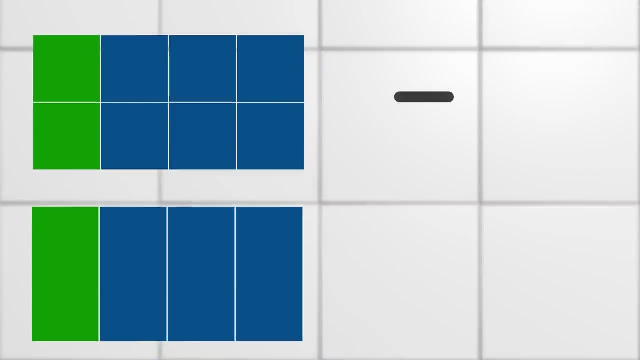 differently. Let's write the fractions for these rectangles and start with the top one. The denominator shows the total amount of parts. So how many pieces is the rectangle cut into Eight pieces? Good job, Now for the numerator. We want to know how many pieces are colored green. 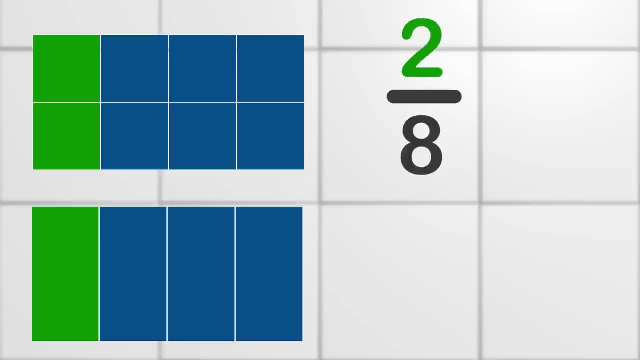 There are two pieces. Our fraction is two-eighths. Can you tell me what the fraction is for the bottom rectangle? The fraction is one-fourth. Great job, Did you notice that the pieces in this rectangle are different than the rectangle above it? 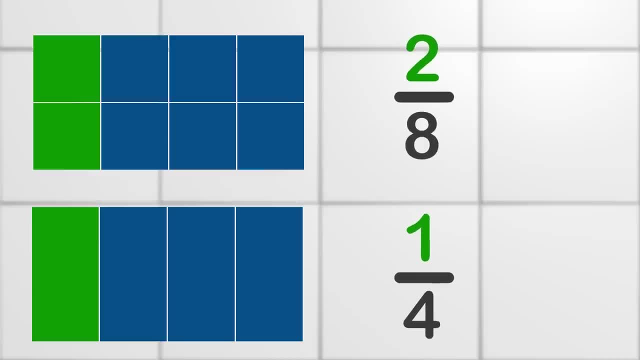 Let's look at these two fractions. We have two-eighths and one-fourth. They don't look the same, but pay attention to the rectangles. Do the green parts of the rectangle look equal? Yes, you're right, They are equal. These two fractions are equivalent fractions. The amount: 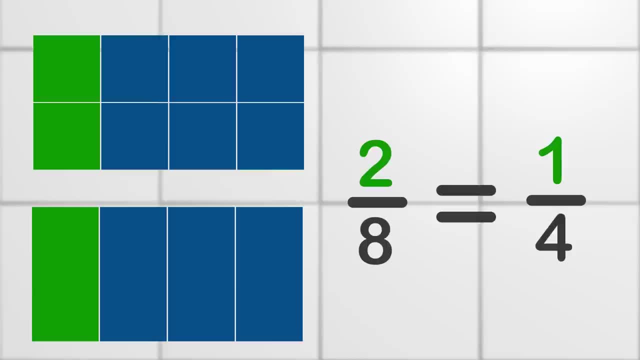 colored green is the same amount. Even though the numerators and denominators are different, the fractions are the same or equal to each other, which make two-eighths and one-fourth equivalent fractions. Let's take a look at another math concept. This is fun stuff. 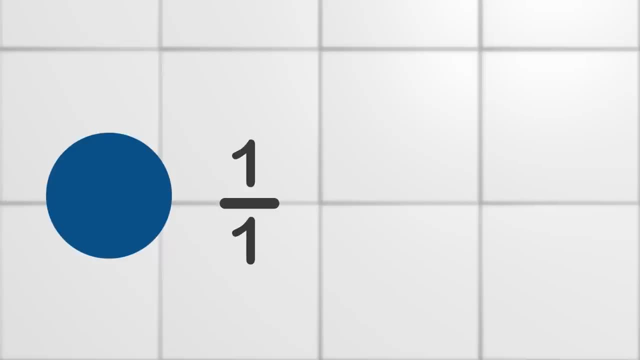 Here we have one whole circle and the fraction one over one. This might seem strange, because there is one complete circle with no separate parts colored. Should this really be just the number one, Or is one over one correct? The answer is: both are correct. One over one is the same. 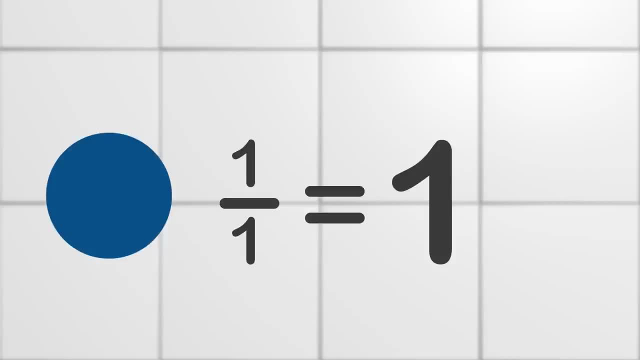 as saying the whole number one. We have one part over one whole. Look here: This circle is now broken into three equal pieces. The numerator shows all the green parts, which is three, and the denominator shows the total amount of pieces, which is also three. The fraction is still one whole circle. Three-thirds is the same or equal. 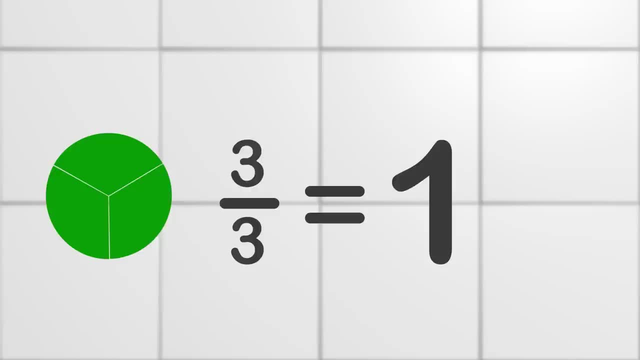 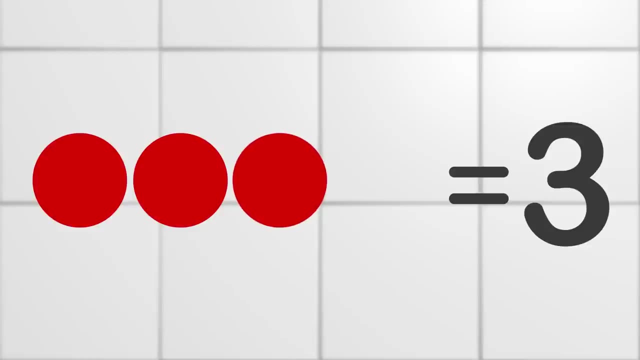 to one. Wow, That is awesome stuff. Now let's look at something really cool. Here we have three circles and we are going to write or express this as a fraction. Here we have a fraction of three over one. This might look kind of weird, because the denominator is smaller than the numerator. 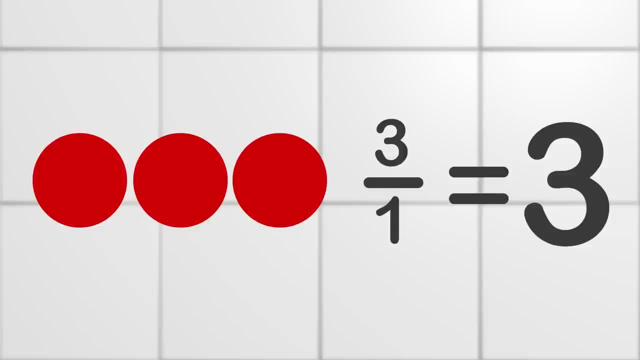 With the earlier problems, we were looking at fractions or parts of one whole. The denominator of one shows the whole cake. We have one whole piece, but the interesting part is that we have three whole cakes and that is why the numerator shows three. So three over one is equal to the whole number three. 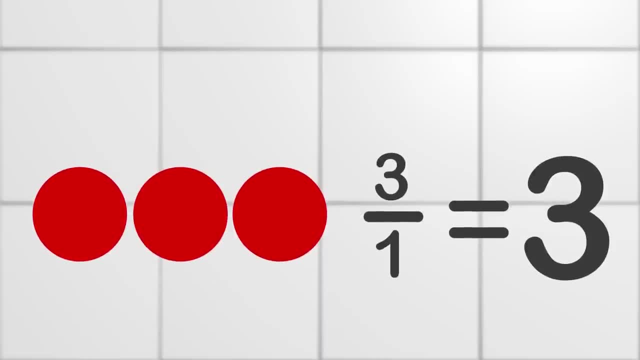 You might be thinking that is kind of hard to understand. Shouldn't the fraction be three over three, because there are three whole circles? Well, that is not true, because we just learned that three over three is the same or equal to one. So in order to write three whole circles into a fraction, you would write three over one. 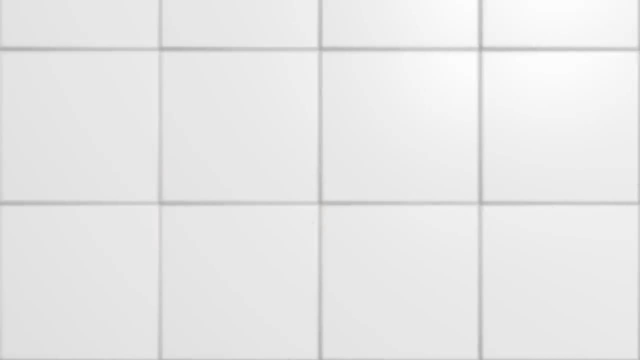 Great job. Let's take a look at a problem you might encounter. Here we have the fraction on the left. one half is equal to blank over four. We need to find the numerator that goes in the empty box. There are different ways you can do this, but I want to use a drawing. 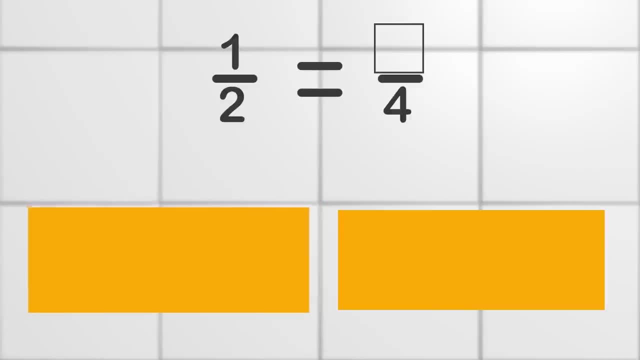 Here are two rectangles. The rectangle on the left will be the one representing the one half. To make the rectangle represent one over two, we need to divide it into two pieces, because the denominator is two. The one green part is the number one in the numerator. 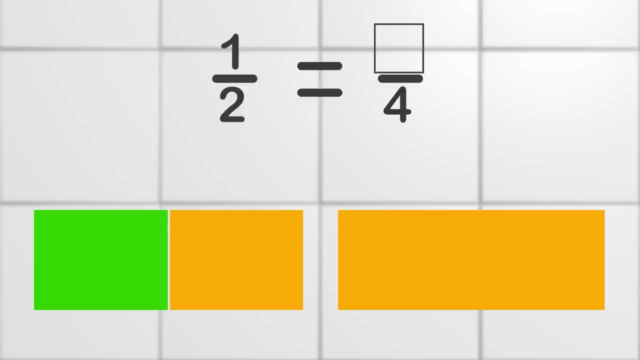 We now have represented the fraction one-half The rectangle on the right. we don't know what the numerator will be, but we do know that the fractions are equal because of the equal sign. So let's start by making the rectangle look like the fraction on the left.